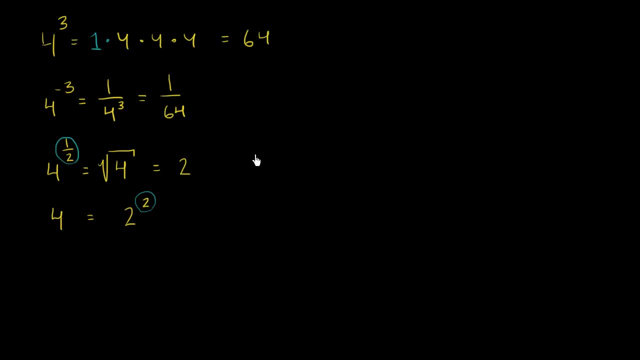 And I encourage you to pause it as much as necessary and try to figure it out yourself. So, based on what I just told you, what do you think 9 to the 1 half power is going to be? Well, that's just the square root of 9.. 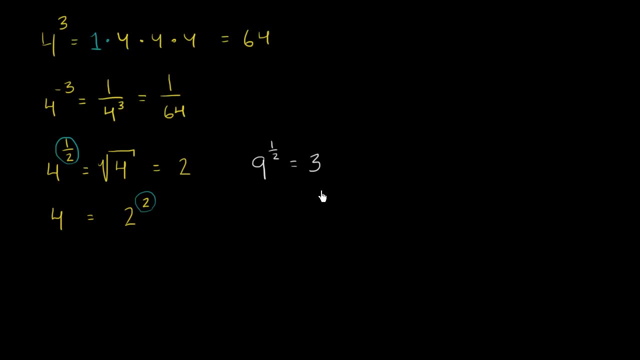 The principal root of 9,. that's just going to be equal to 3.. And likewise we could have also said that 3 squared is, or let me write it this way- that 9, 9 is equal to 3 squared. 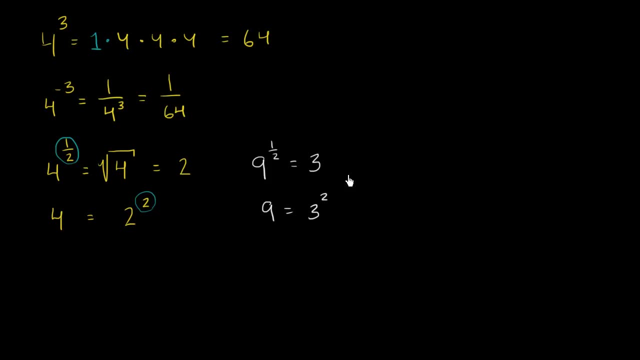 These are both true statements. Let's do one more like this: What is 25 to the 1 half going to be? Well, this is just going to be 5.. 5 times 5 is 25.. Or you could say that 25 is equal to 5 squared. 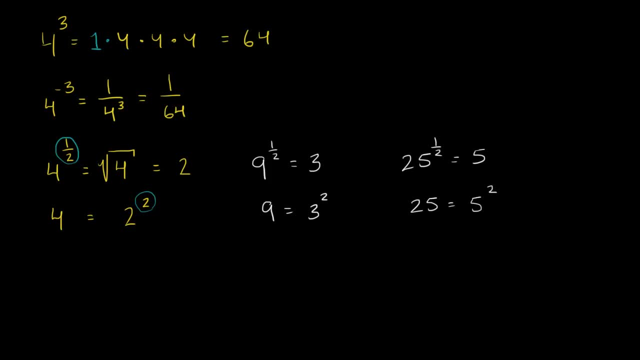 Now let's think about what happens when we take something to the 1 third power. So let's imagine taking 8 to the 1 third power. So the definition here is that taking something to the 1 third power is the same thing. 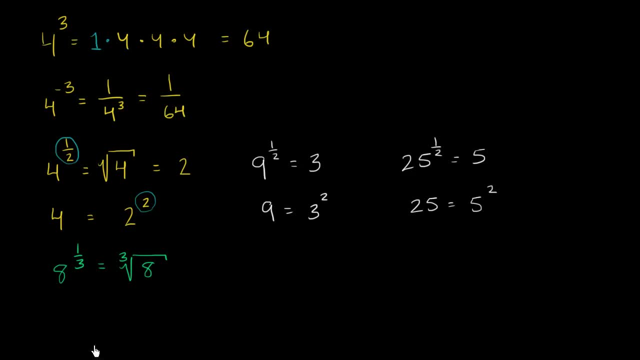 as taking the cube root of that number. And the cube root is saying: well, if I had 3 of that number and I multiply them that I'm going to get 8.. So something times something times something is 8.. Well, we already know that 8 is equal to 2. to the third power. 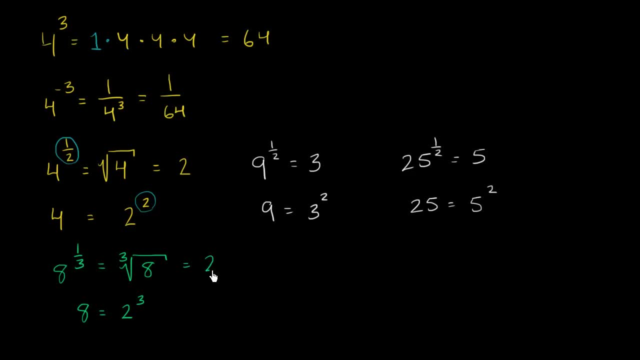 So the cube root of 8, or 8 to the 1 third, is just going to be equal to 2.. This says: hey, give me the number that if I say that number times that number, times that number, I'm going to get 8.. 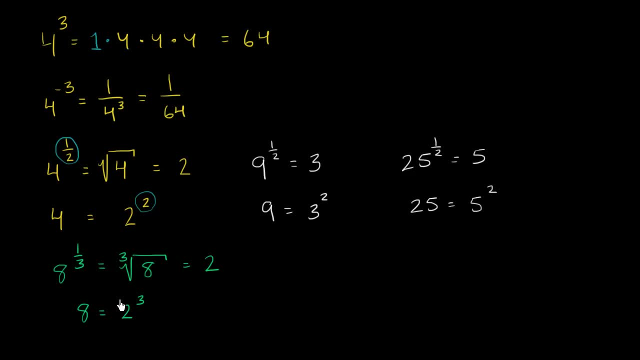 Well, that number is 2, because 2 to the third power is 8.. Do a few more examples of that. What is 64 to the 1 third power? Well, we already know that 4 times 4 times 4 is 64.. 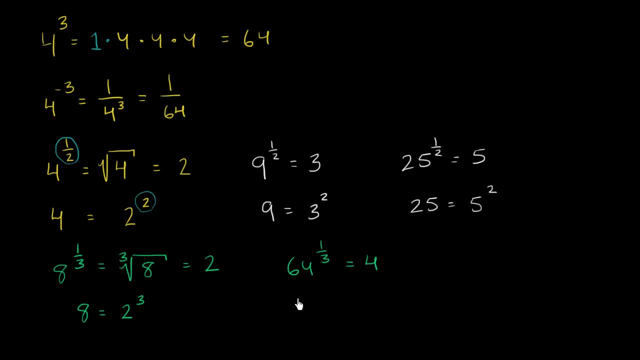 So this is going to be 4.. And we already wrote over here that 64 is the same thing as 4. to the third. I think you're starting to see a little bit of a pattern here, a little bit of symmetry here.